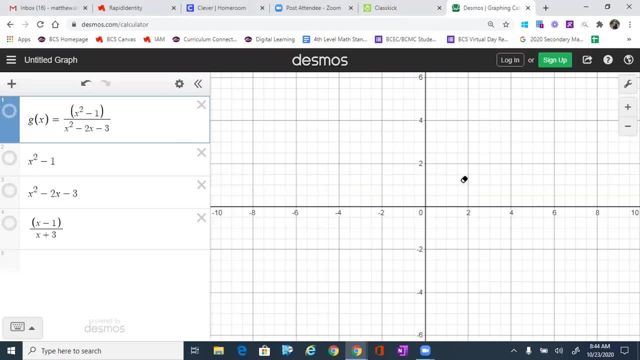 to go to Desmos and factor this. We can use the area model, but I'm going to go to Desmos because these have a leading coefficient of one, So they're nice and easy to get done. So when I turn on x squared minus one, you're going to notice that we have a negative one as a root. 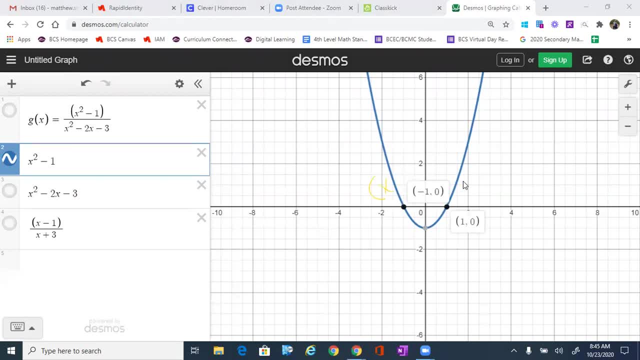 positive one as a root, and we can go ahead and write our factors as x plus one, x minus one, And so let's go back to our class kick and let's clear that out, And I'm going to write that in the. 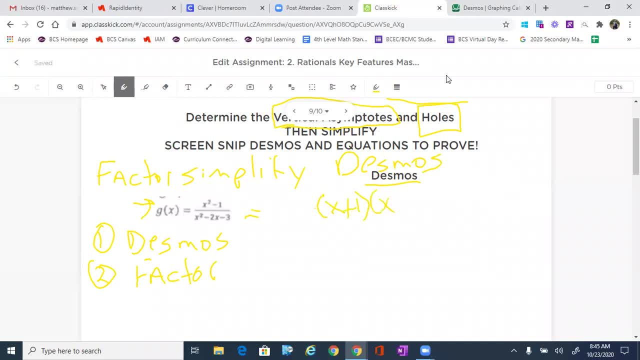 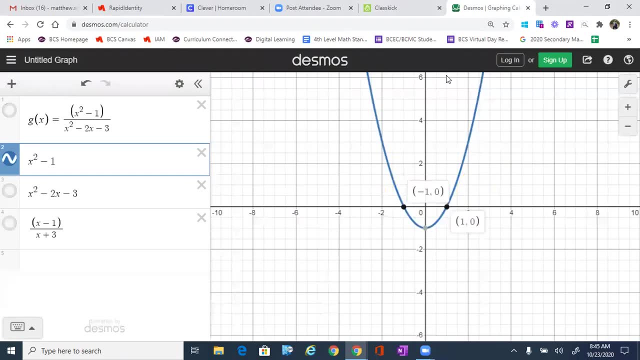 numerator. So x plus one and x minus one. Now I'm going to do the same thing. I'm going to find my. I'm going to factor x squared minus two, x minus three in Desmos as well. Turn this one off. 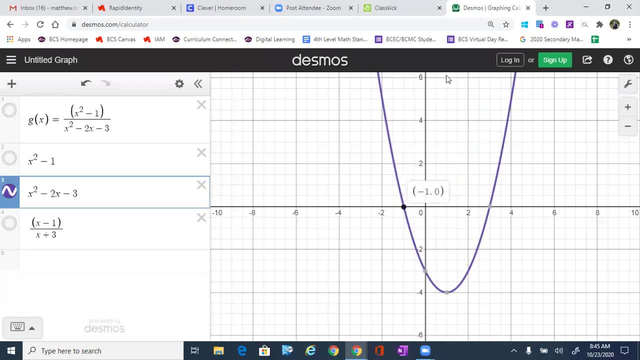 and let's go to the other one. You'll notice that we have x minus one and x I mean negative one and positive three, which means we're going to have the factors of x plus one and x minus three. 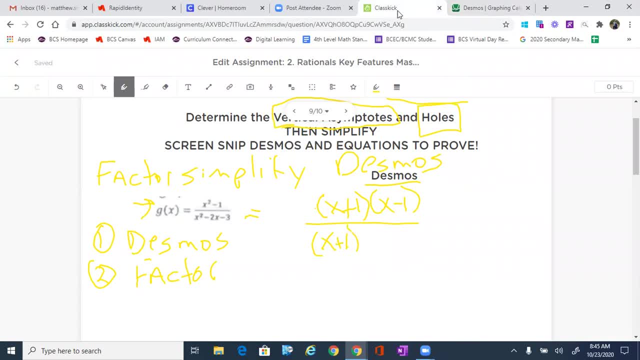 So I'm going to do that, I'm going to write x plus one and x minus three, x minus three. Now remember, we take those x intercepts, we put them in as opposites, and then we will make those factors nice and easy. Okay, so number three. once you've got it factored. 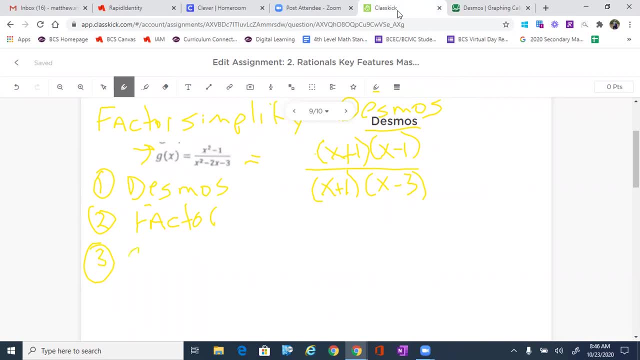 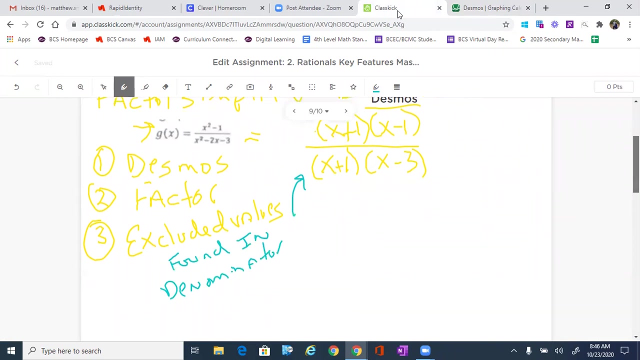 we are going to find the excluded values. okay, Remember, excluded values are found in the denominator. okay, So, right there, found in denominator, Denominator, Denominator. And the reason why they're excluded values is because we cannot divide by zero. So cannot divide by zero, We're not going to. we're going to get an undefined. 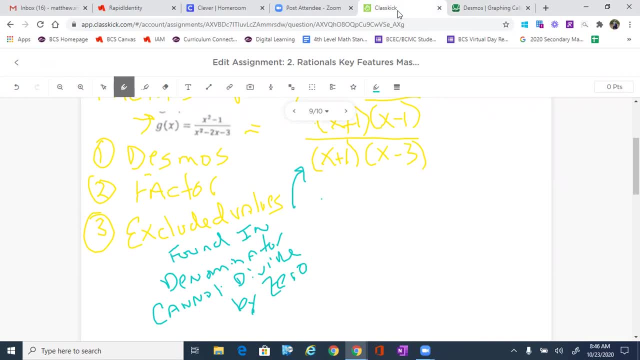 answer. if that's the case, So all we have to do is come up here and say: well, what does x have to be in order for that value right here to be zero? Well, if I put negative one in, I get negative. one plus one which is zero. So I'm going to put negative one in and I get negative one plus one which is zero. So I'm going to put negative one in and I get negative one plus one which is zero. 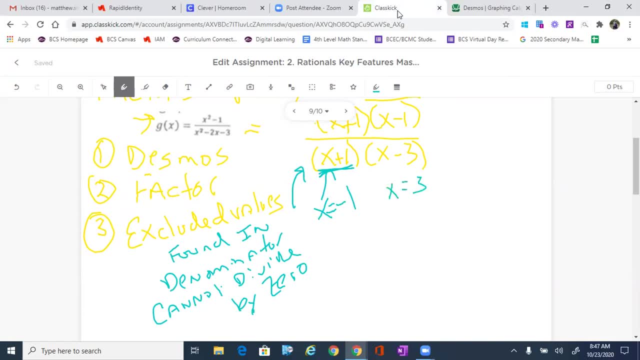 zero. And then if I put an x equals to three in this statement, that would give us a zero. So these guys right here are our excluded. Okay, in our domain, negative one and three cannot exist. Let's check it on Desmos. Okay, so we go to Desmos. I'm going to go to that graph which I've got. 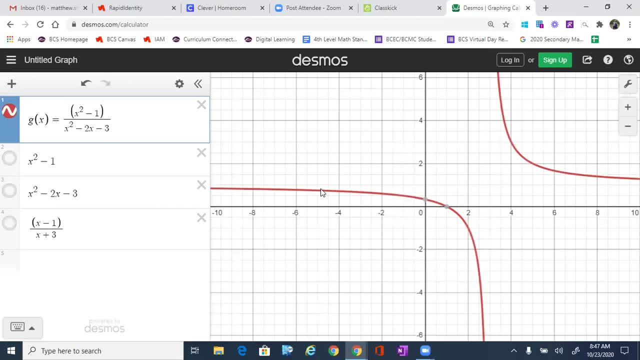 typed in here to save us a little bit of time And I'm going to drag it along And I'm going to look for negative one And check it out. negative one on our graph is undefined. You'll also notice check out on Desmos. it does a great job of showing us a circle that is not filled in that. 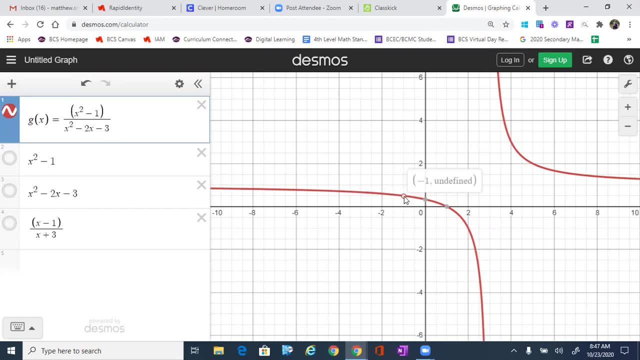 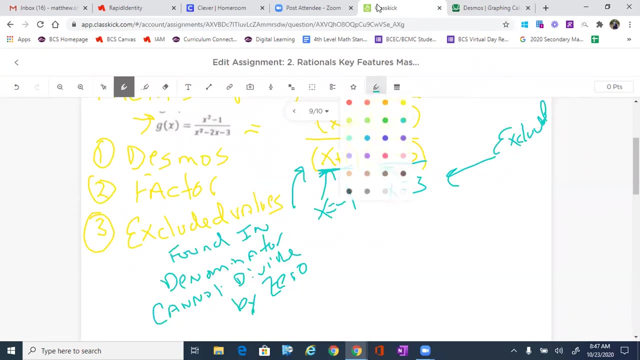 tells us it is not included And there's not a distinct break. it is just a hole. And we can tell it's a hole because it's a circle with an empty, an empty circle in the graph and not a distinct break. So I'm going to come back to my class, kick right here And I'm going to say, Hey guys, we just 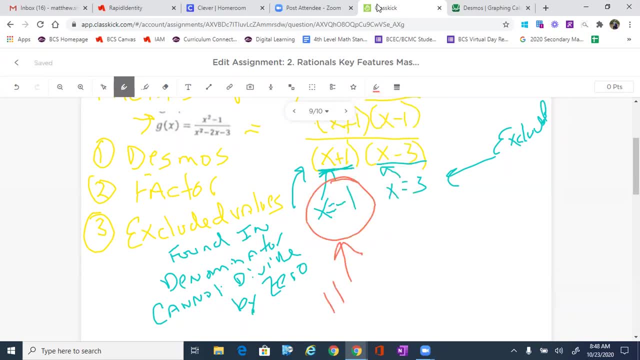 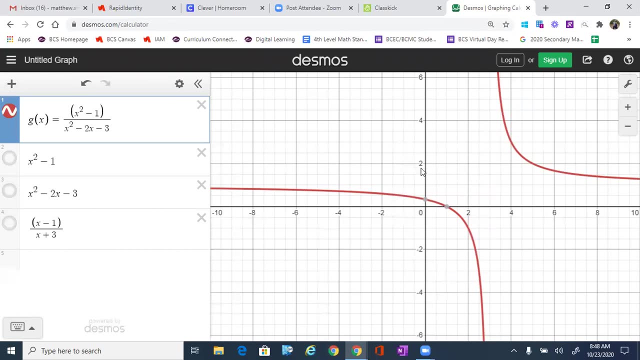 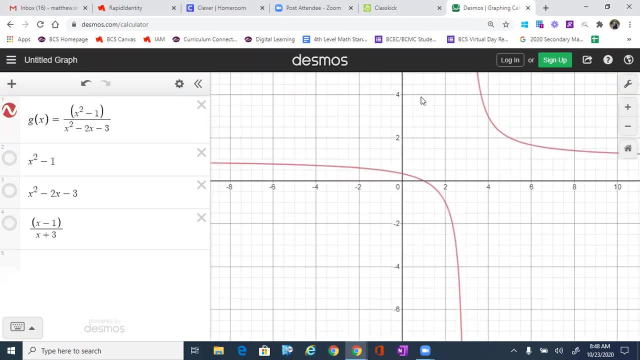 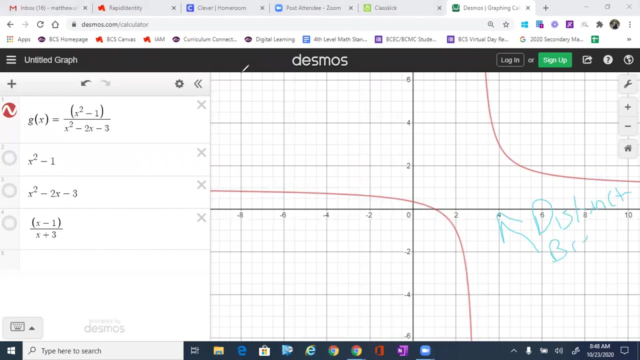 figured out: x equals negative one. that's a hole, Okay. And then I'm going to go over to x equals to three. Let's check out that graph right there, x equals to three. Well, if I take a moment and just look at the peer, there is a distinct graph break. So there is a distinct break, Okay. and 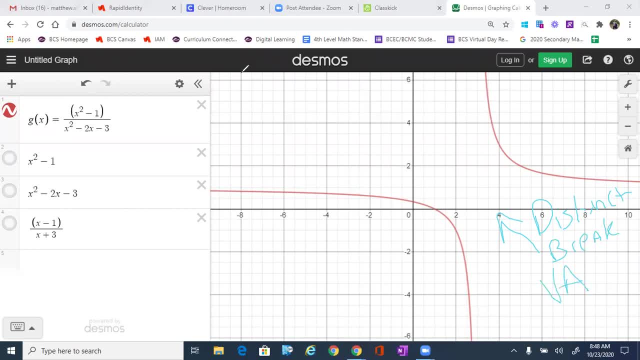 that distinct break is a hole. So I'm going to go over to my class kick right here And I'm going to check out that graph right there. Okay, and that distinct break is our vertical asymptote And I just have to figure that out. So let's go ahead here. Let's go and say, Okay, well, where is that? 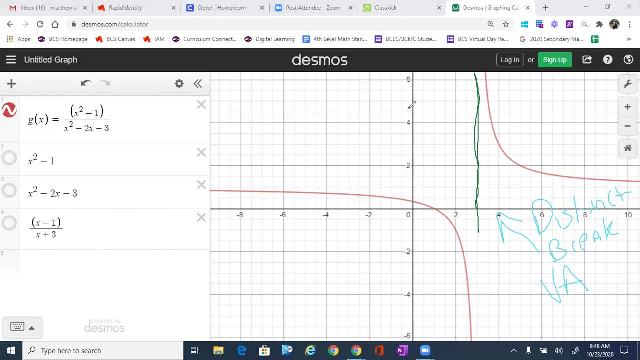 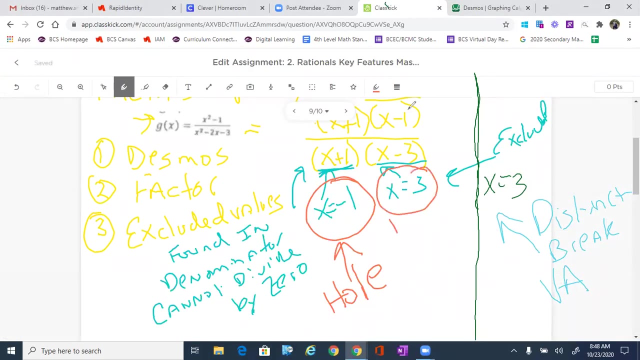 distinct break. Well, check it out right here. I go up And I go down at x equals to three. That's your distinct break, That is your vertical asymptote. So I'm going to go back here. Let's go ahead and identify that. I'm going to say: x equals to three is our vertical asymptote. Woo Now. 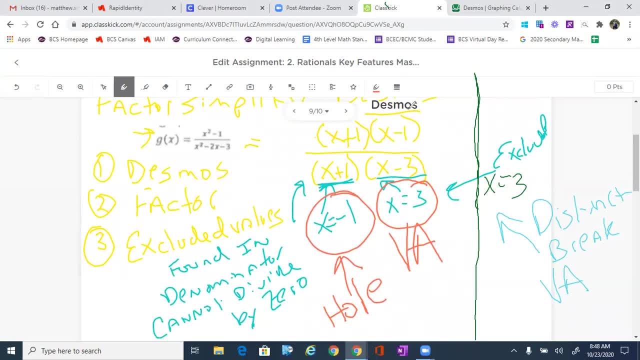 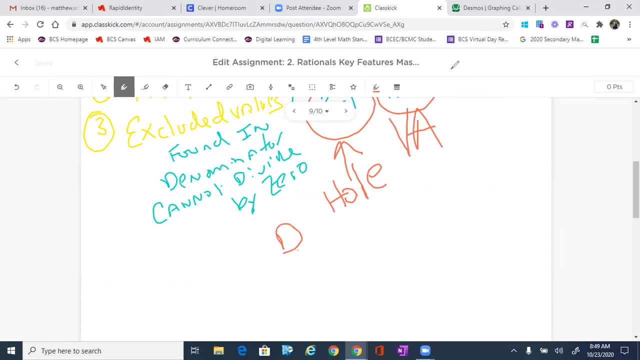 how can we find that on a from our factors? Okay, so that's what we need to know. How do we find it from the, from the equation, determine from equation or the function? Okay, Well, let's go back up here The first thing I want to write. 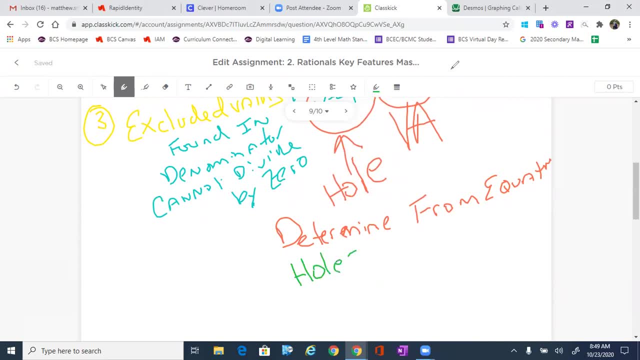 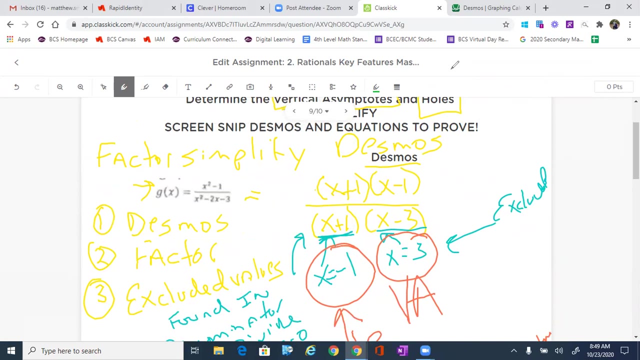 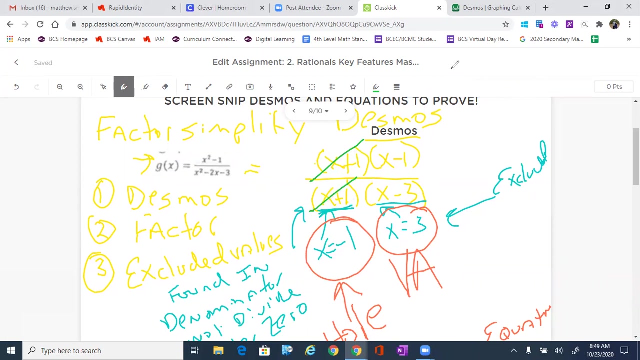 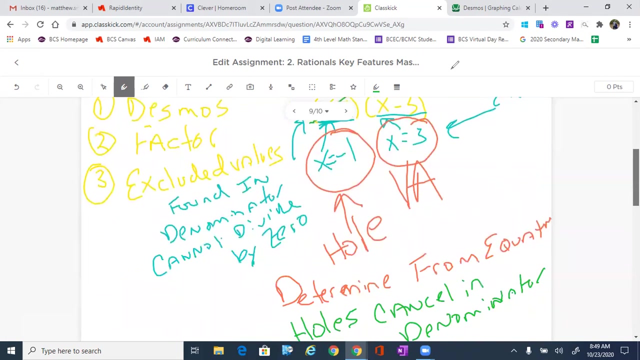 down is holes Cancel In denominator Completely, not just one, but they completely cancel in the denominator. Notice that we said the hole was negative one. Well, that's because x plus one cancels with x plus one. There are no more x plus ones in the denominator. That gives us a hole. Okay, Vertical asymptotes. 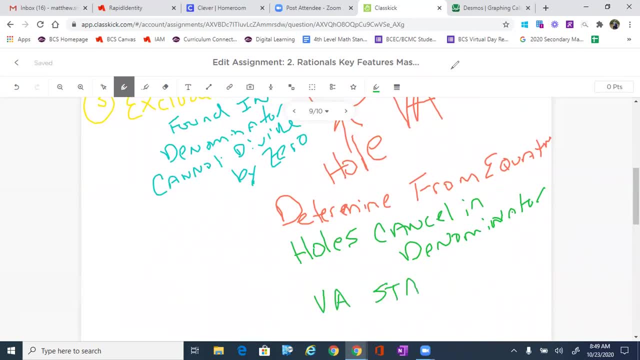 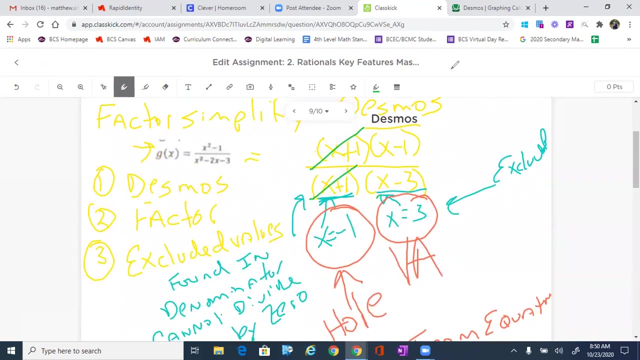 stay in the denominator, Even if you cancel a bunch of them out. If there's still one in the denominator, it's going to create a vertical asymptote. Okay, now check it out: x minus one. x minus three cannot cancel because there's none x minus three up at the top. We have fully simplified this: x plus one. x plus one cancels out and we are left with this statement: x minus one. 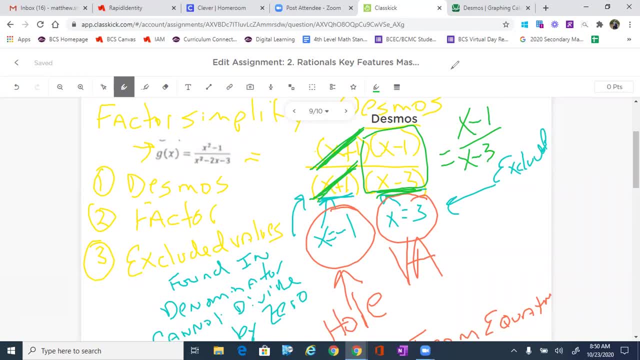 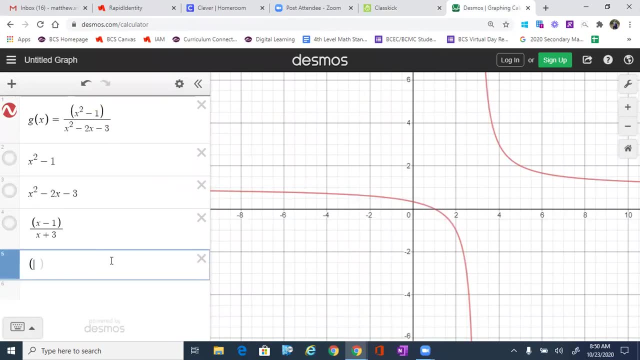 Over: x minus three minus three. So now how do we even check if we've done the simplification correctly? I'm going to go over to Desmos. I am going to type that beast in, So let's go over here. I'm going to write x minus. 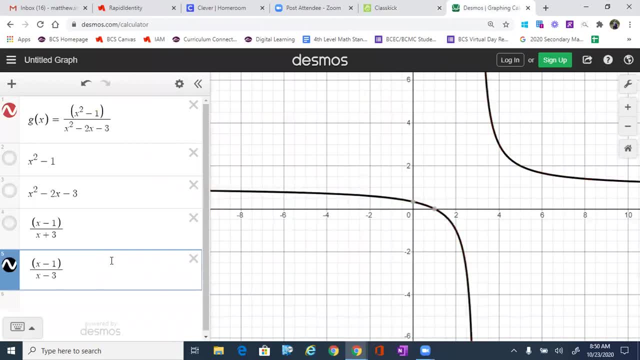 one. I'm going to divide it by x minus three. Bada, boom, bada bing. Check it out. If we've done it correct, they are equivalent. They are equivalent, which means their graphs are going to overlap. So we've simplified the whole. We determined, We found the whole. We determined the vertical. 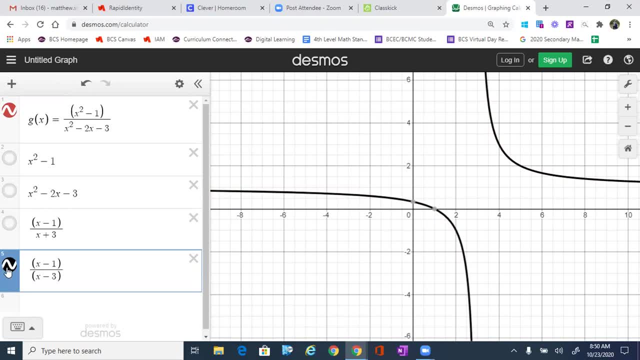 asymptote as a break in the graph, and we went ahead of schedule and we went ahead and simplified that rational function. I hope you all enjoyed it. Y'all have a great day. It's beautiful. 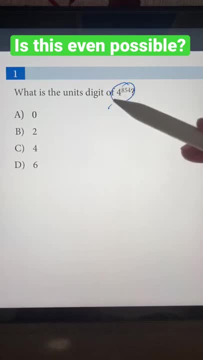 What is the units digit of 4 to the power of 854?? So, first of all, this number is so big you can't even put in a calculator, but let's see if we can find some sort of pattern. So 4 to the 1 power is: 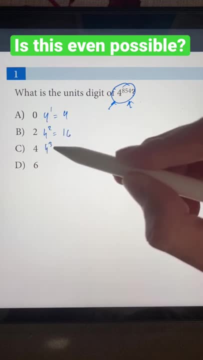 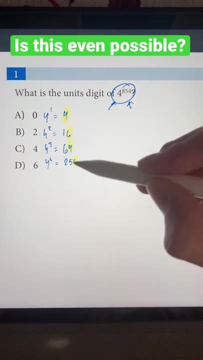 just 4.. 4 squared is just 16.. 4 to the 3rd power is just 64.. 4 to the 4th power is 256.. So, as you can see in the ones digit it goes from 4 to 6 to 4 to 6, and it repeats like that forever. 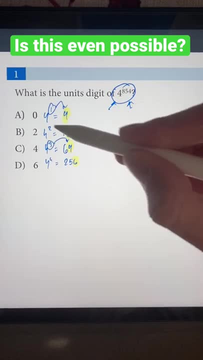 And every time we have an odd power, it goes to a 4.. And every time we have an even power, it goes to a 6.. So since 854 is an even number, it's going to go to a 6,, which means the answer.